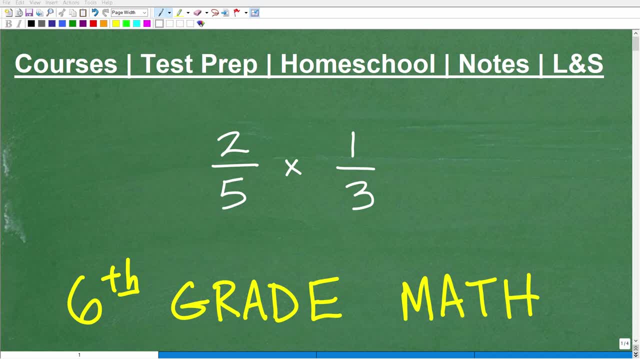 Okay, let's talk about how to multiply fractions, And this is definitely something that you need to know if you're at the sixth grade level or beyond. Now, fractions is a huge topic in all levels of mathematics. Even in elementary school, you start learning basic concepts of fractions. 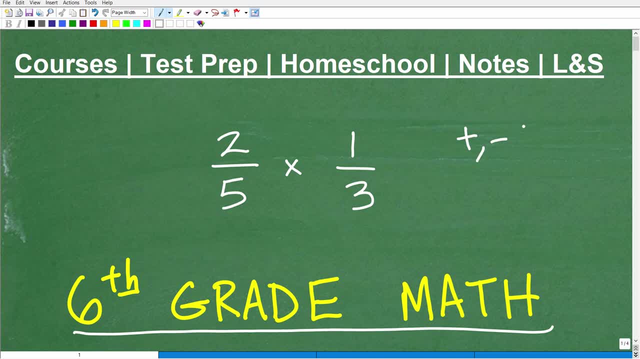 But when you're in middle school, you definitely need to know how to add, subtract, multiply and divide fractions, along with other things, And the easiest thing to do when it comes to fractions by far is to multiply fractions, okay, So if I would have to kind of classify this or 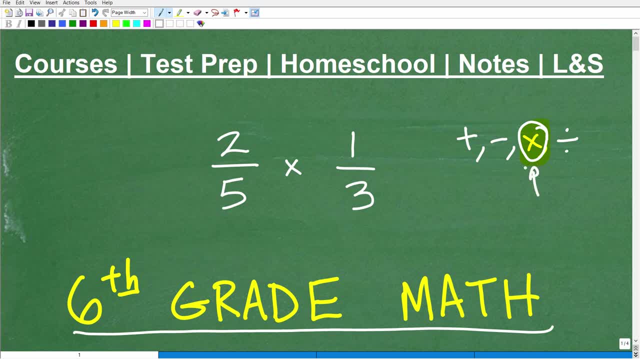 order these things in terms of difficulties. the easiest thing to do is to multiply fractions. The second easiest thing to do is to divide fractions And then adding and subtracting fractions. this is also not that difficult, but this is where you have to deal with the LCD. 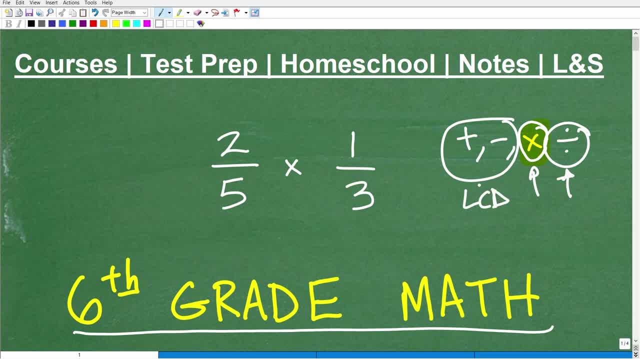 And this is typically where students just like- oh, they just, you know, fall apart. They hate fractions, They don't want to deal with fractions. get that Way back in the good old days when I was in middle school, elementary school. 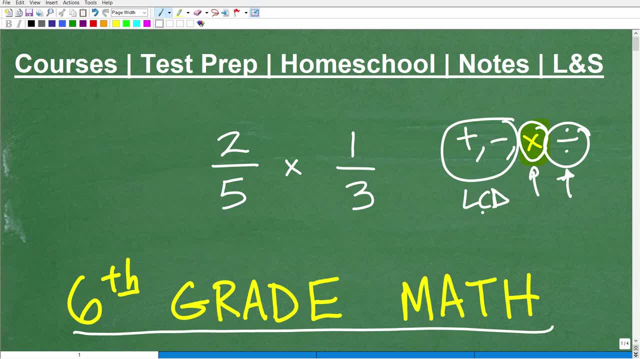 probably even high school. I didn't like dealing with fractions either, But you need to know how to work with fractions. They are everywhere in mathematics at all levels. So let's go ahead and review how to multiply fractions- Super easy. but we'll take a look at a couple of variations. 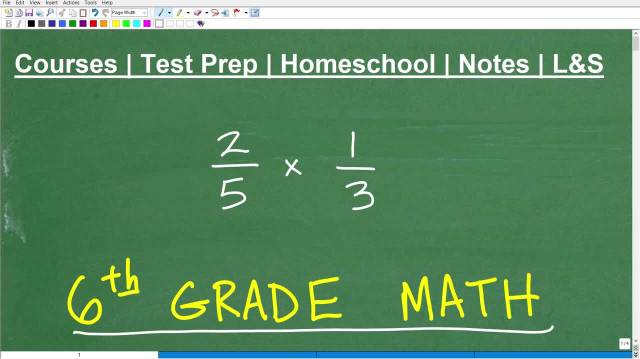 and some additional points that I want to make that are related to multiplying fractions, Some other things that we need to be thinking about as well, But we're going to get into all this in just one second. But first, let me quickly introduce myself. My name is John. I'm the 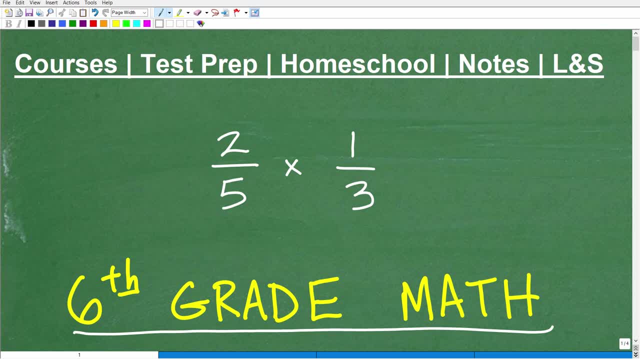 founder of TC Math Academy. I'm also a middle and high school math teacher. I've been teaching math for decades And I'm telling you right now: if you're struggling in mathematics, there is hope. So don't give up. To be successful in mathematics, the main thing you need is great math instruction. 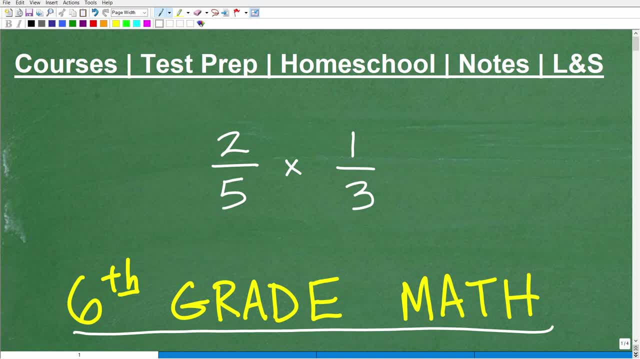 Hopefully you've got an excellent math teacher, But if you need additional help in math, I can help you out with clear, understandable, comprehensive mathematics For those of you who are at the middle school, high school or even college level. 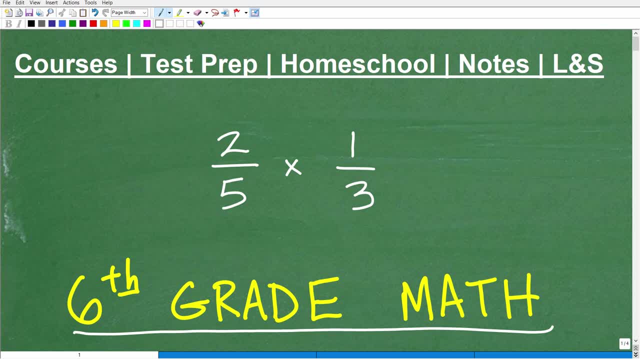 founder of TC Math Academy. I'm also a middle and high school math teacher. I've been teaching math for decades And I'm telling you right now: if you're struggling in mathematics, there is hope. So don't give up. To be successful in mathematics, the main thing you need is great math instruction. 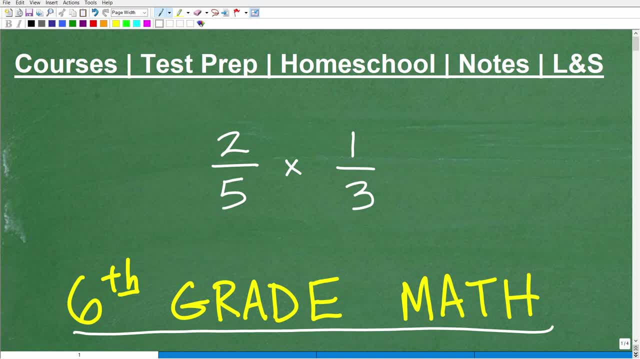 Hopefully you've got an excellent math teacher, But if you need additional help in math, I can help you out with clear, understandable, comprehensive mathematics For those of you who are at the middle school, high school or even college level. 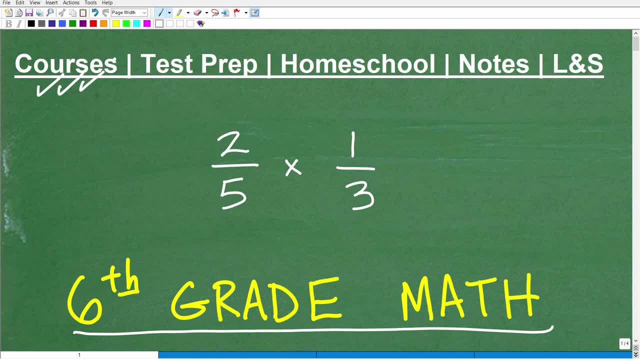 check out my math help program. You can find a link to it in the description of this video. I promise you it will help you out big time in your respective studies Now, if you happen to be preparing for some sort of test that has a dedicated math section. there's a lot of them. 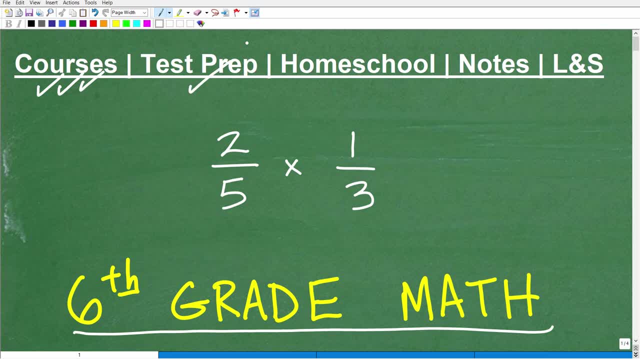 things like the GED, SAT, ASVAB, ACT, GRE, GMAT, maybe a teacher certification exam. I can help you out. If you homeschool, I have excellent homeschool math courses for middle and high school mathematics. If you need a pair of math notes, I'm going to leave links to my math notes in the description. 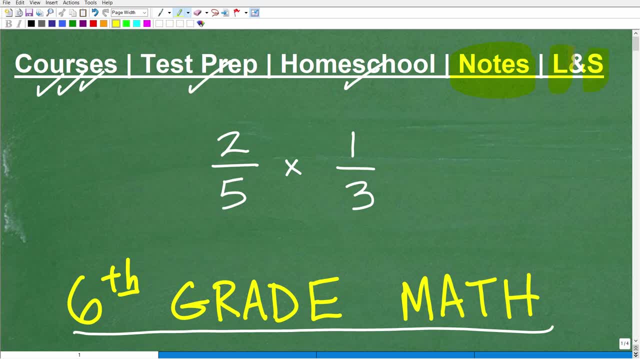 of this video, And if this video helps you out, don't forget to help me out by liking and subscribing to my channel. That would be much appreciated. So now let's get into how to multiply fractions, And if you want to play along, go ahead and tell me the answer, If you know. 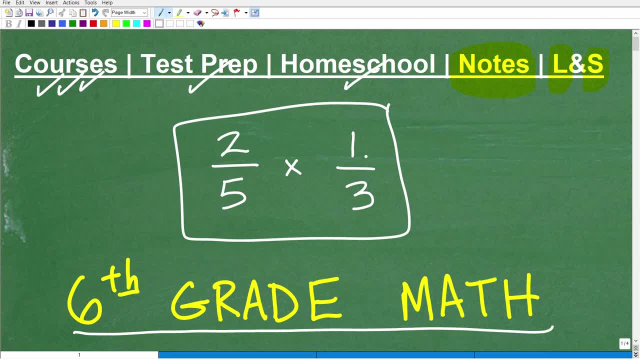 how to multiply two-fifths times one-thirds. of course I'm going to cover this here in just one second. I'll put the answer to that in the comment section. But here's the deal. Don't guess. Okay. Now, if you have to take a guess, that's fine, But that's the thing with. 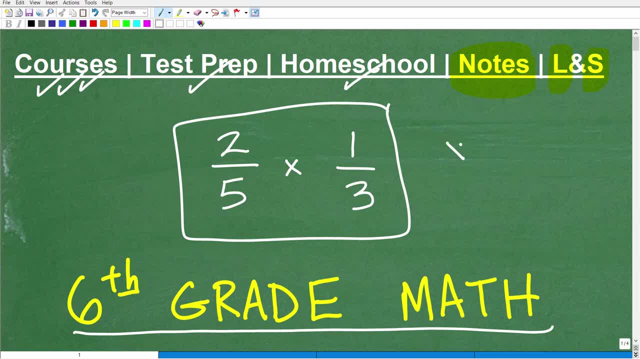 fractions. Students confuse. you know how to multiply and divide, add and subtract. They'll like: oh yeah, I think I do this. You don't want to be thinking anything, You just want to be absolutely positive on how to do these operations. So let's get into it right now And we'll actually. 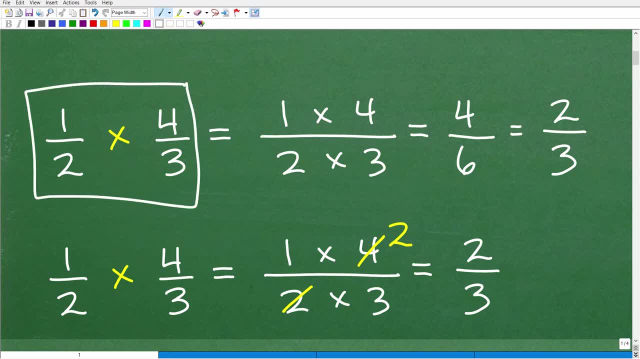 do this problem here. Okay, One-half times four-thirds. So how do you multiply fractions? Well, here is the deal. It is super easy. What you're going to do is you're going to multiply the respective numerators. The numerator is the top number, Okay, So basically, you're just going to multiply. 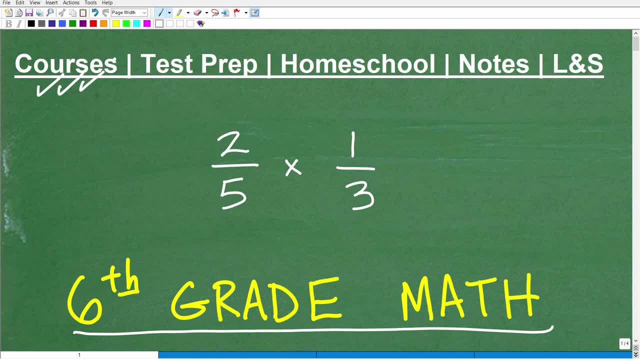 check out my math help program. You can find a link to it in the description of this video. I promise you it will help you out big time in your respective studies Now, if you happen to be preparing for some sort of test that has a dedicated math section. there's a lot of them. 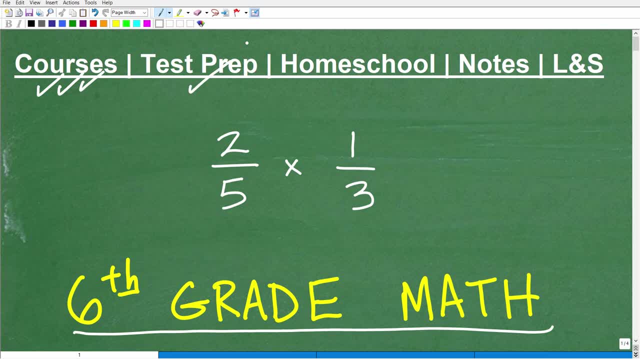 things like the GED, SAT, ASVAB, ACT, GRE, GMAT, maybe a teacher certification exam. I can help you out. If you homeschool, I have excellent homeschool math courses for middle and high school mathematics. If you need a pair of math notes, I'm going to leave links to my math notes in the description. 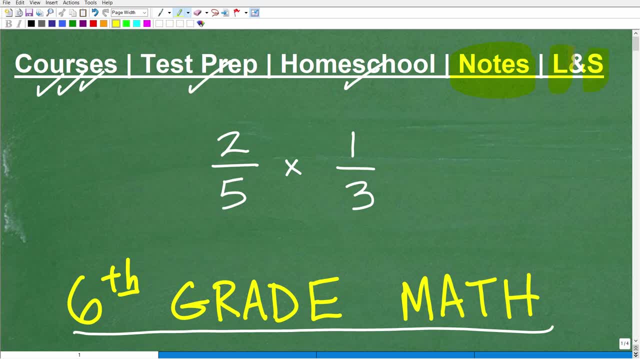 of this video, And if this video helps you out, don't forget to help me out by liking and subscribing to my channel. That would be much appreciated. So now let's get into how to multiply fractions, And if you want to play along, go ahead and tell me the answer, If you know. 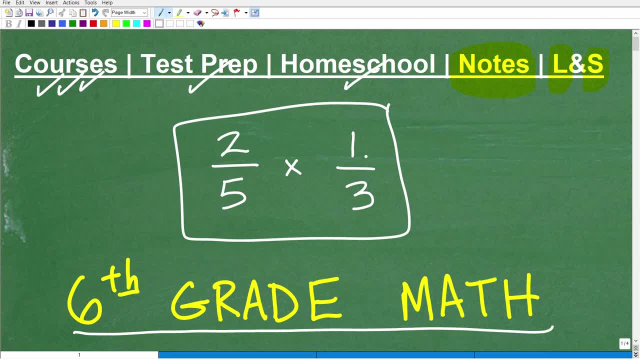 how to multiply two-fifths times one-thirds. of course I'm going to cover this here in just one second. I'll put the answer to that in the comment section. But here's the deal. Don't guess. Okay. Now, if you have to take a guess, that's fine, But that's the thing with. 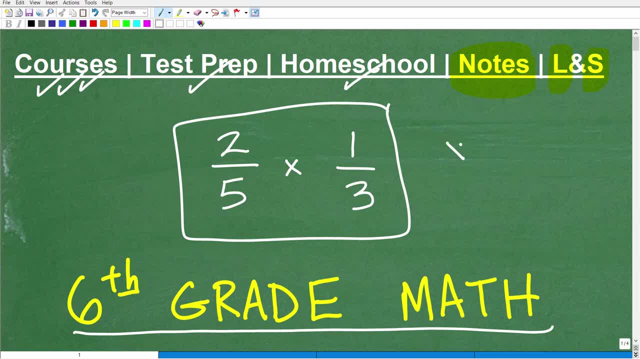 fractions. Students confuse. you know how to multiply and divide, add and subtract. They'll like: oh yeah, I think I do this. You don't want to be thinking anything, You just want to be absolutely positive on how to do these operations. So let's get into it right now And we'll actually. 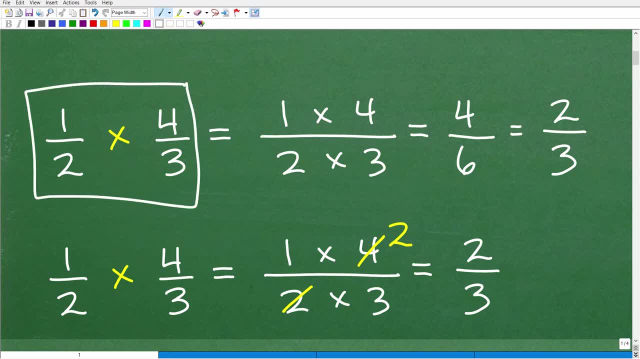 do this problem here. Okay, One-half times four-thirds. So how do you multiply fractions? Well, here is the deal. It is super easy. What you're going to do is you're going to multiply the respective numerators. The numerator is the top number, Okay, So basically, you're just going to multiply. 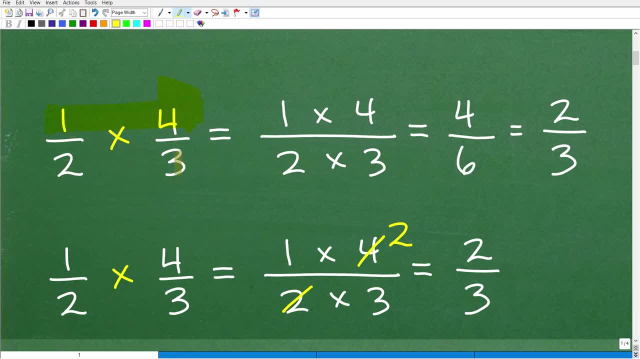 across. So here we have one-half times four-thirds. The numerators is one and four, So we're going to multiply across. That'll be our numerator And then our denominator. we're just going to multiply the respective denominators or the bottom numbers, So two. 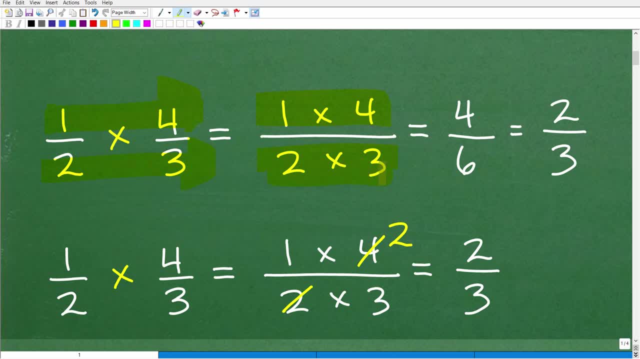 times three is going to be two times three. That's going to be our answer for our denominator, And one times four will be our answer for our numerator. So when we're finding the product of one-half times four-thirds, all we do is simply multiply across. And now let's go ahead. 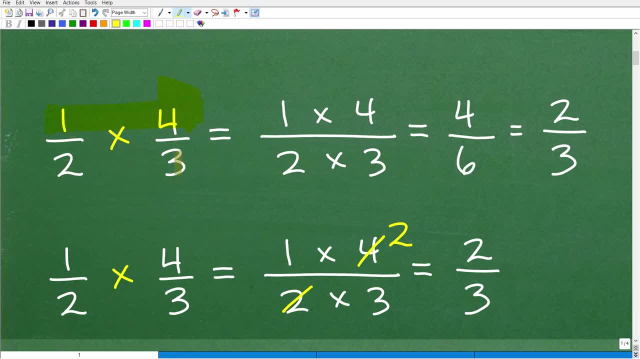 across. So here we have one-half times four-thirds. The numerators is one and four, So we're going to multiply across. That'll be our numerator And then our denominator. we're just going to multiply the respective denominators or the bottom numbers, So two. 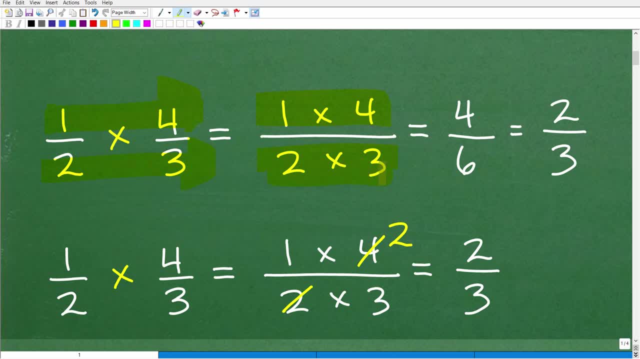 times three is going to be two times three. That's going to be our answer for our denominator, And one times four will be our answer for our numerator. So when we're finding the product of one-half times four-thirds, all we do is simply multiply across. And now let's go ahead. 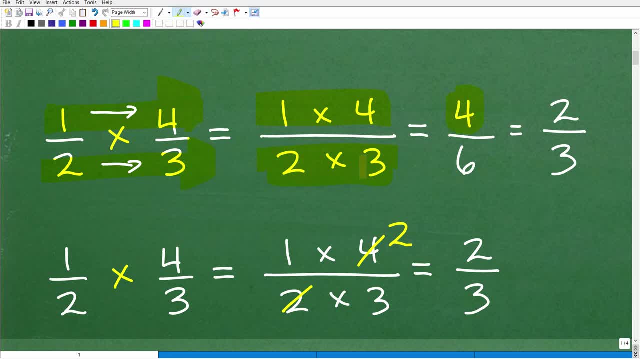 and figure this out. So one times four is, of course, four, Two times three is six. But here is the deal. Okay, You never just multiply fractions together and just stop. You always need to ask yourself: is your fraction fully simplified? Is it really simplified? Is it really simplified, Is it? 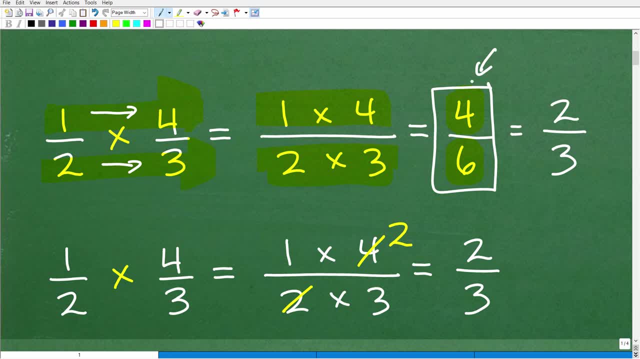 reduced 100%. If you left your answer just like this, a lot of math teachers will take points off, as they should, because you need to know how to simplify and reduce. Of course, that's a separate discussion. But four is six is equal to, or can be reduced to, the fraction two-thirds, So always. 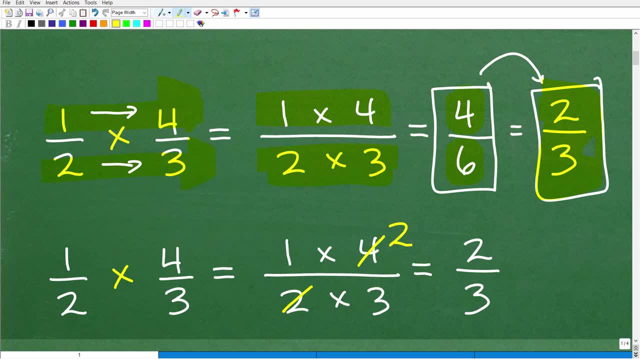 leave your answer in its most simplified manner. Now let's take a look at the same problem and talk about how you can kind of reduce or simplify Your answer as you do your multiplication. So here we go. We got one-half times four-thirds I. 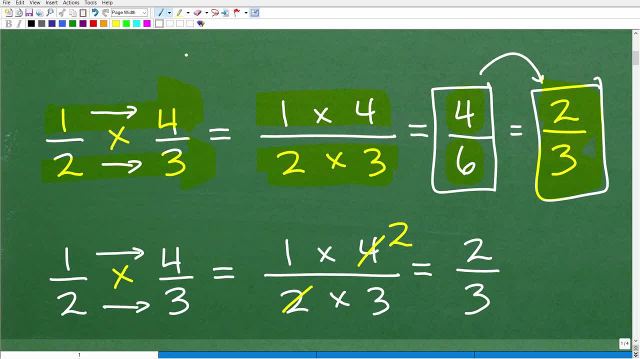 already talked about to multiply fractions. you're going to multiply the respective numerators and denominators, So here this is going to be one times four, Okay, And then our denominator will be two times three. Now you can see, I'm doing something right here, And what I'm doing is: 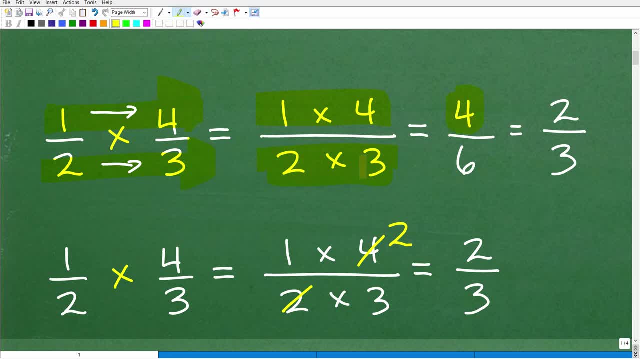 and figure this out. So one times four is, of course, four, Two times three is six. But here is the deal. Okay, You never just multiply fractions together and just stop. You always need to ask yourself: is your fraction fully simplified? Is it really simplified? Is it really simplified, Is it? 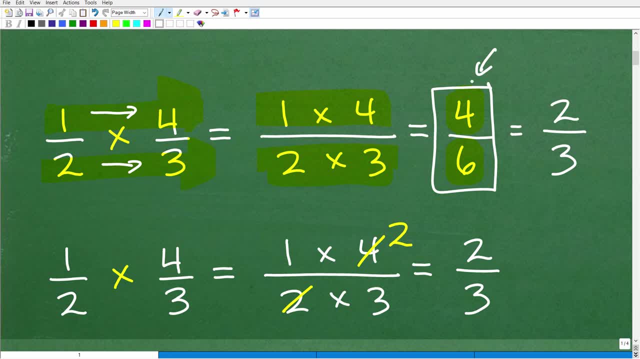 reduced 100%. If you left your answer just like this, a lot of math teachers will take points off, as they should, because you need to know how to simplify and reduce. Of course, that's a separate discussion. But four is six is equal to, or can be reduced to, the fraction two-thirds, So always. 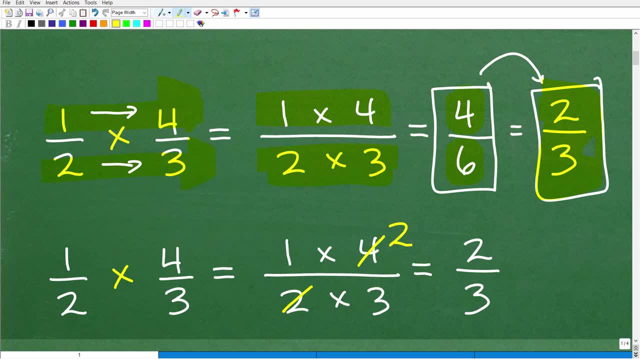 leave your answer in its most simplified manner. Now let's take a look at the same problem and talk about how you can kind of reduce or simplify Your answer as you do your multiplication. So here we go. We got one-half times four-thirds I. 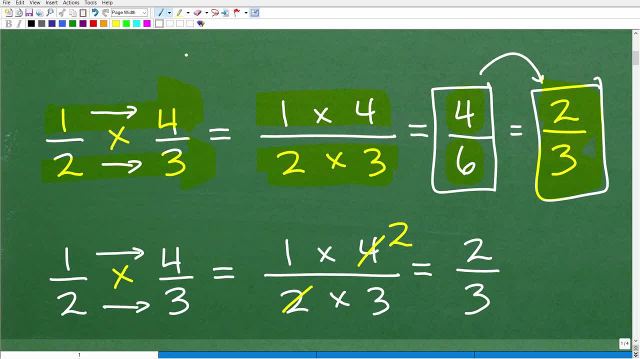 already talked about to multiply fractions. you're going to multiply the respective numerators and denominators, So here this is going to be one times four, Okay, And then our denominator will be two times three. Now you can see, I'm doing something right here, And what I'm doing is: 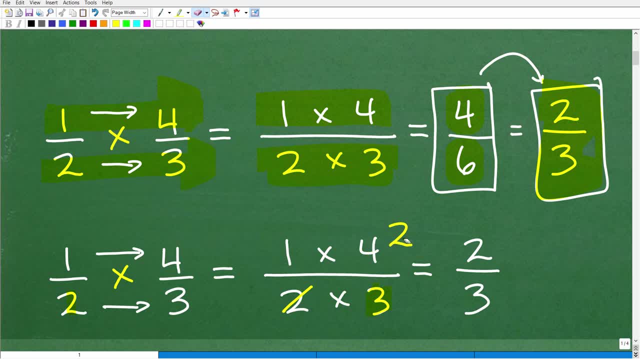 called cross-canceling. Okay, Now let me show you exactly what's going on. Okay, So four. all right, we can think of four as two times two. Okay, That is four, And all these things, all these numbers are being separated by multiplication. That means that these are: 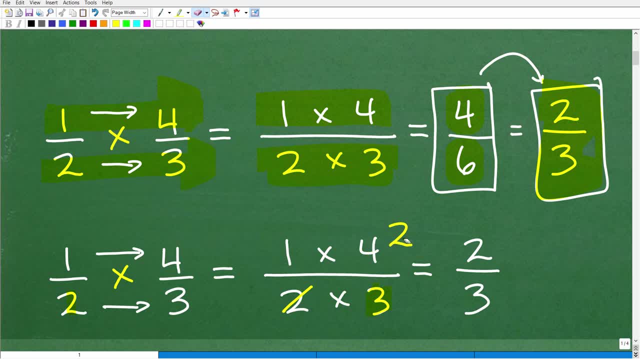 called cross-canceling. Okay, Now let me show you exactly what's going on. Okay, So four. all right, we can think of four as two times two. Okay, That is four, And all these things, all these numbers are being separated by multiplication. That means that these are: 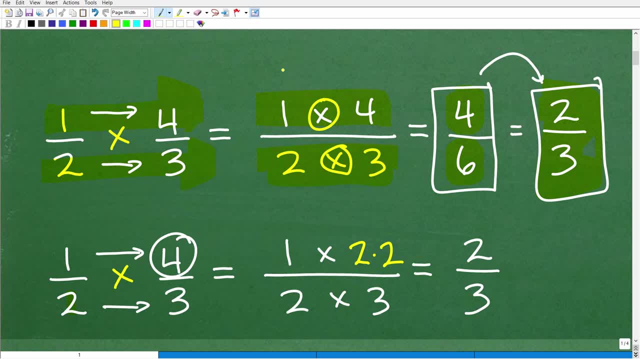 factors. Okay, So in math when you have a like factor, in other words you have the same factor in the numerator. So in this case, four is two times two. There's a two factor up in the numerator, but I also have a two. 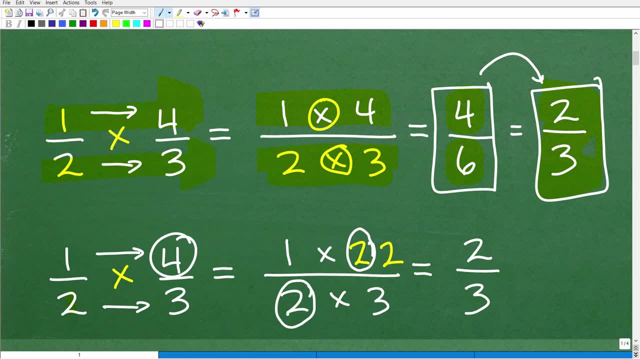 Down here in the denominator, when you have like factors one to one, okay, between the numerator and denominator you can do something called cross-cancel. So basically, this two can divide into that two and that goes away. And now let's take a look at what's left. Okay, What's? 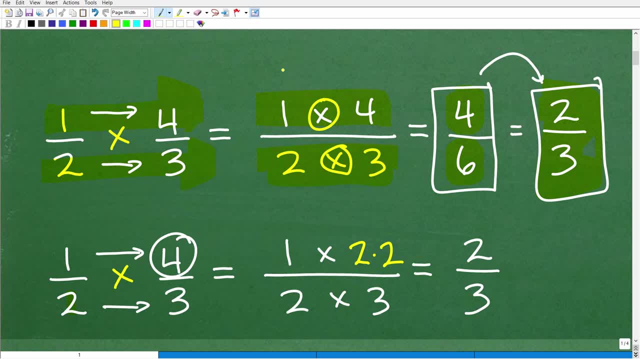 factors. Okay, So in math when you have a like factor, in other words you have the same factor in the numerator. So in this case, four is two times two. There's a two factor up in the numerator, but I also have a two. 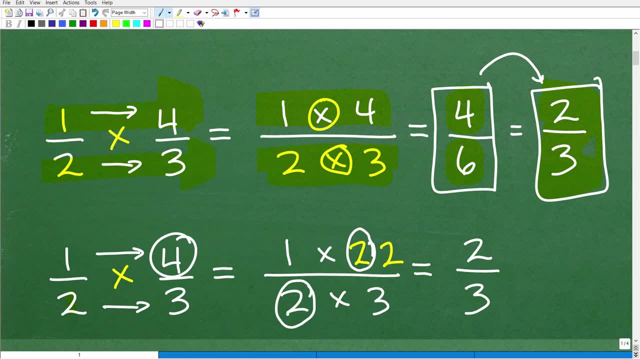 Down here in the denominator, when you have like factors one to one, okay, between the numerator and denominator you can do something called cross-cancel. So basically, this two can divide into that two and that goes away. And now let's take a look at what's left. Okay, What's? 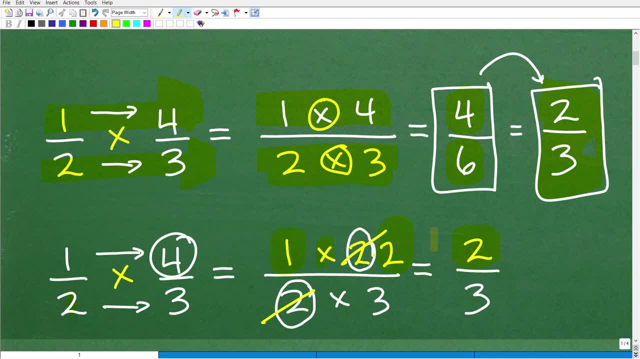 left is one times this two. one times two is two. And then this right here is really just a one, but just one times three. So that is two-thirds And that is our final answer. So you can kind of reduce by cross-canceling as you go. So let me show you this kind of again. 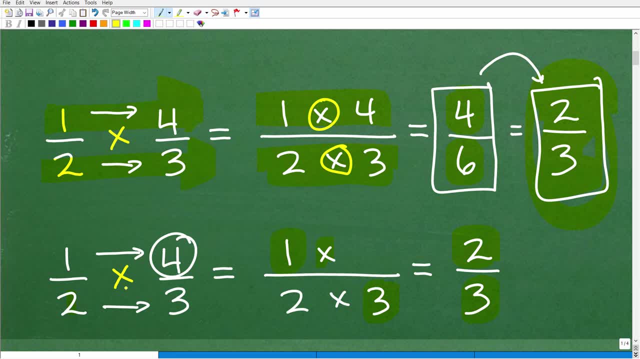 one last time. So here it is One-half times four-thirds, It's one times four, right there. So what you're thinking is: oh, two goes into that four, two. Okay, That's another way to cross-cancel. So now I have one times two is two, And then right here, anytime you cross-cancel, you're really just 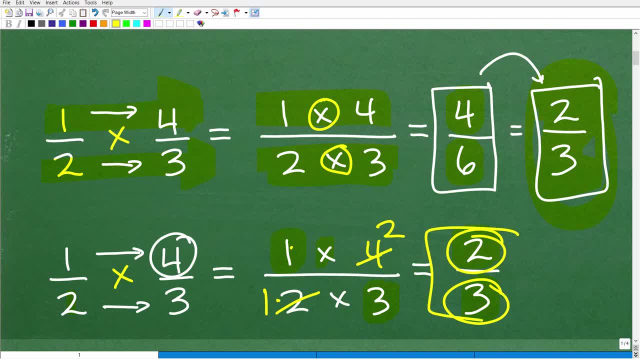 leaving a one behind. So one times three is three. So there is our reduced answer. Or, if you're more comfortable, you can just get your final answer and reduce it this way as well, But you do need to reduce or simplify those fractions, Okay So? 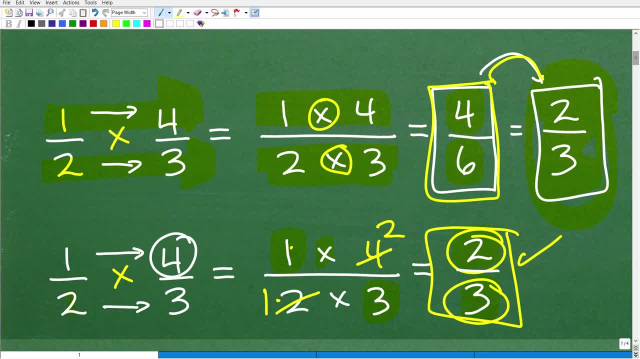 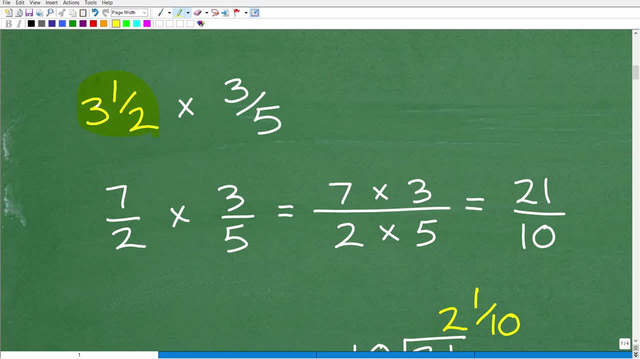 again, multiplying fractions- not that difficult, but let's take a look at some other situations that you're going to be facing And we'll start talking about mixed numbers. So this is a mixed number, Okay, Because it's a whole number with some sort of fraction. So it's like three and 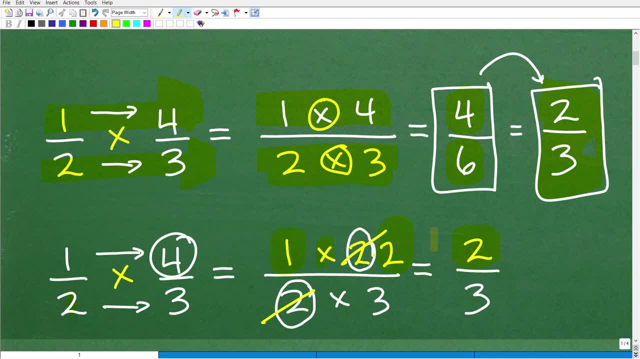 left is one times this two. one times two is two. And then this right here is really just a one, but just one times three. So that is two-thirds And that is our final answer. So you can kind of reduce by cross-canceling as you go. So let me show you this kind of again. 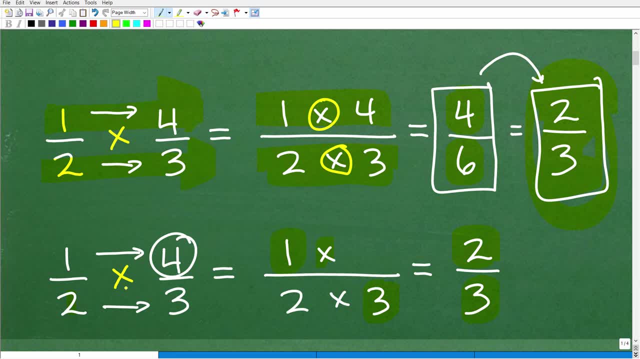 one last time. So here it is One-half times four-thirds, It's one times four, right there. So what you're thinking is: oh, two goes into that four, two. Okay, That's another way to cross-cancel. So now I have one times two is two, And then right here, anytime you cross-cancel, you're really just 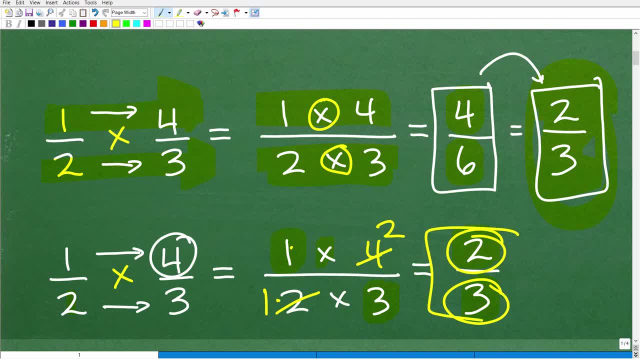 leaving a one behind. So one times three is three. So there is our reduced answer. Or, if you're more comfortable, you can just get your final answer and reduce it this way as well, But you do need to reduce or simplify those fractions, Okay So? 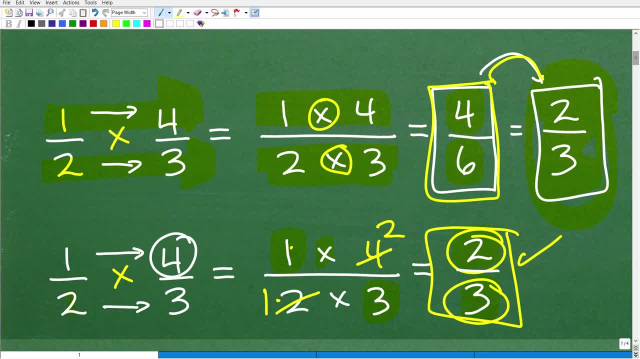 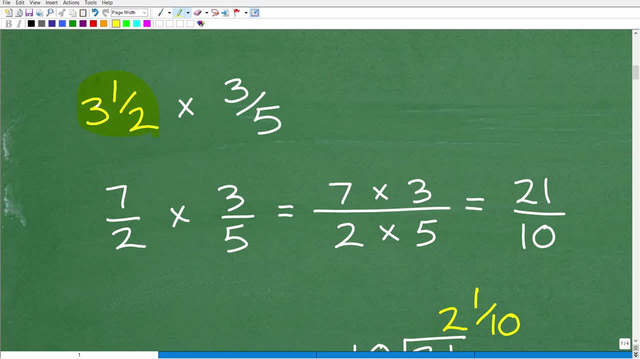 again, multiplying fractions- not that difficult, but let's take a look at some other situations that you're going to be facing And we'll start talking about mixed numbers. So this is a mixed number, Okay, Because it's a whole number with some sort of fraction. So it's like three and 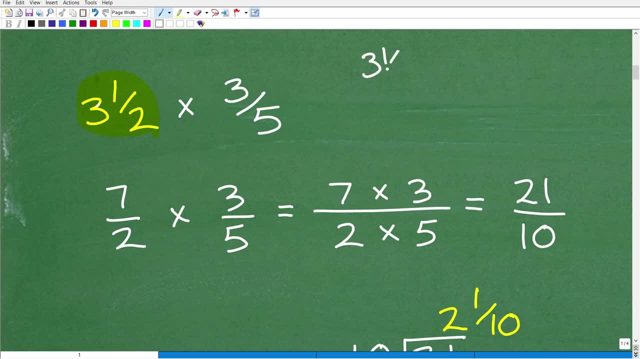 one-half. We've classified this. It has a mixed number. Matter of fact, let's just do a quick view. This is a mixed number fraction. A fraction like three-fifths is a proper fraction because the denominator that bottom number is. 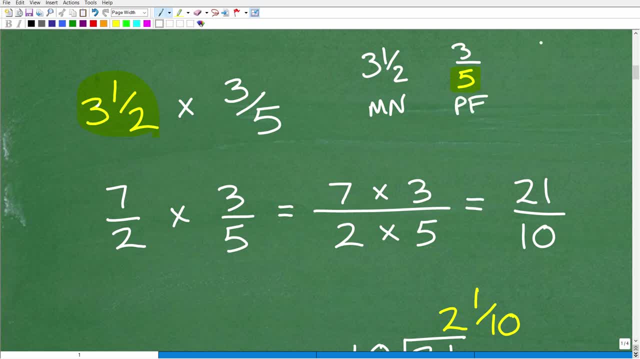 larger than the numerator. So this is a proper fraction. And then if the numerator- that top number- is bigger than the bottom number, this is called an improper fraction. Okay, So you do need to be familiar with these terms So we can convert mixed number fractions into improper fractions, And you need to know how to do. 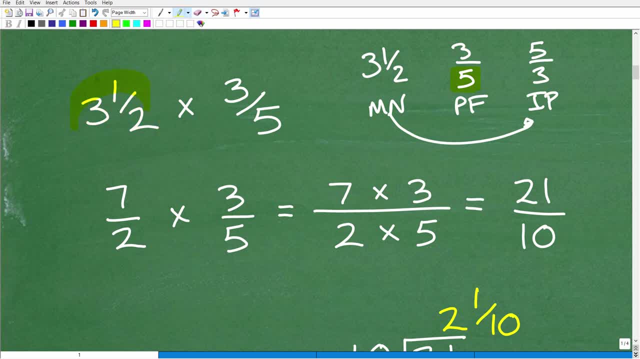 that And, matter of fact, we're going to discuss that right now. So when we want to multiply two fractions and one of those fractions is a mixed number, fraction one or both, okay, you need to convert all mixed number fractions into improper fractions. So let's do this now. So how do I do? 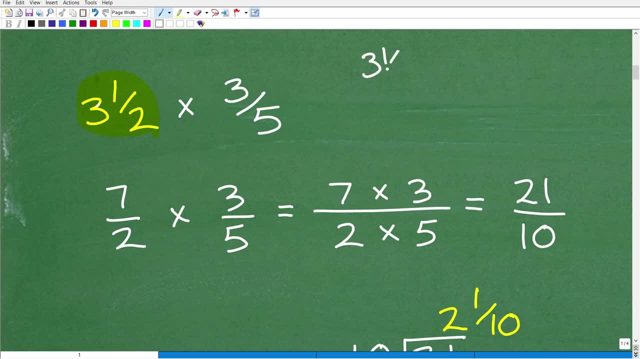 one-half. We've classified this. It has a mixed number. Matter of fact, let's just do a quick view. This is a mixed number fraction. A fraction like three-fifths is a proper fraction because the denominator that bottom number is. 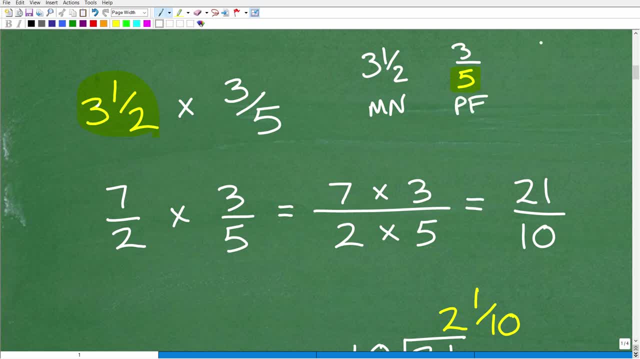 larger than the numerator. So this is a proper fraction. And then if the numerator- that top number- is bigger than the bottom number, this is called an improper fraction. Okay, So you do need to be familiar with these terms So we can convert mixed number fractions into improper fractions, And you need to know how to do. 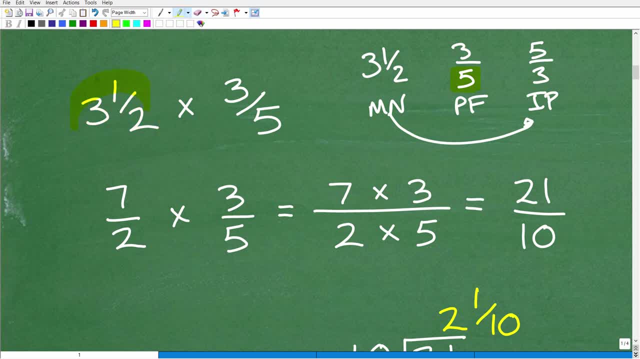 that And, matter of fact, we're going to discuss that right now. So when we want to multiply two fractions and one of those fractions is a mixed number, fraction one or both, okay, you need to convert all mixed number fractions into improper fractions. So let's do this now. So how do I do? 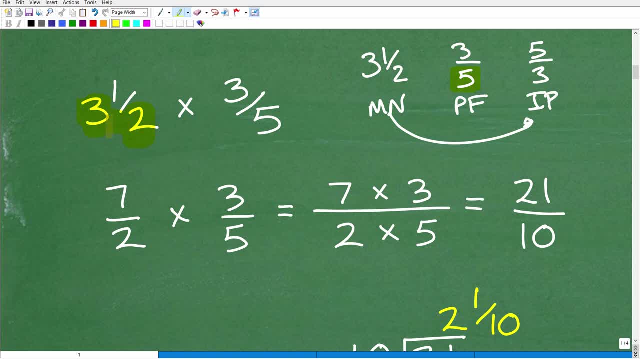 that. Well, you take this two, you multiply by that three, So two times three is six plus one. Okay. So six plus one is seven, over that little denominator right there. So that's seven halves, Okay. So if you need additional help on fractions, how to write mixed number fractions as improper? 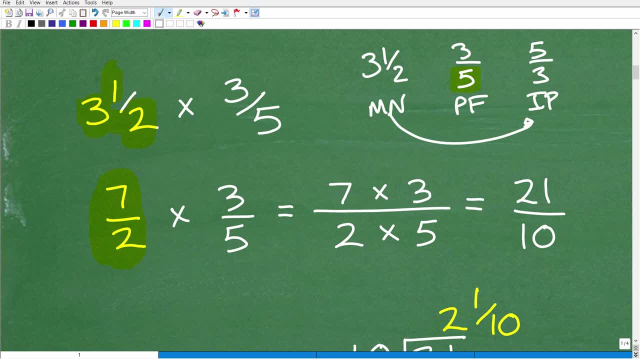 fractions. I have additional videos on this. I teach all of this in my pre-algebra course and my math foundation course. You can check those out by just going to my math help program. But let's go ahead and keep this problem going. So the first thing you're going to do, 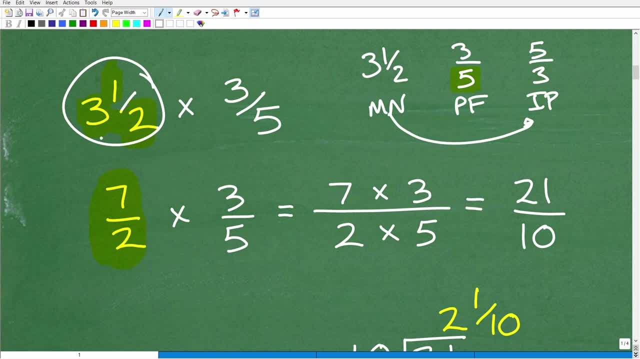 is you're going to multiply the number fractions into improper fractions. So that's going to be seven halves times our three fifths. So now we have one numerator, one denominator. one numerator, one denominator, And at this point we're good to go to go ahead and actually multiply the. 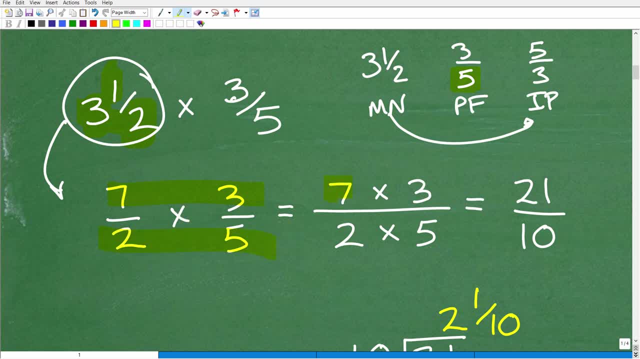 respective numerators and denominators. So seven times three. always write your factors out like this And I'm going to show you why here in a second: So seven times three. just don't answer that. It's going to be like: oh, seven times three is 21.. Show your work for. 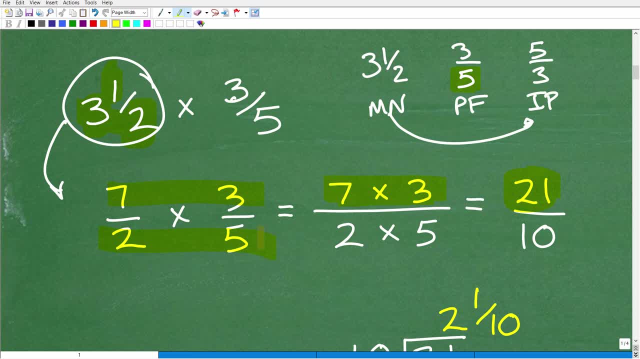 your teacher. But there's another reason here. in a second I'll show you. Of course, two times five is 10.. But you want to write it like this, because here I have seven times three and two times five. The reason why you want to write out all your factors here is because you want to look for. 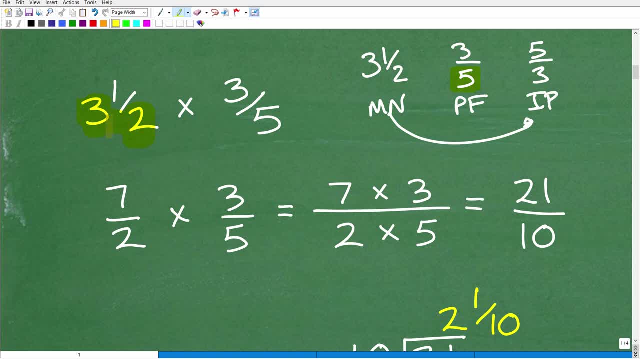 that. Well, you take this two, you multiply by that three, So two times three is six plus one. Okay. So six plus one is seven, over that little denominator right there. So that's seven halves, Okay. So if you need additional help on fractions, how to write mixed number fractions as improper? 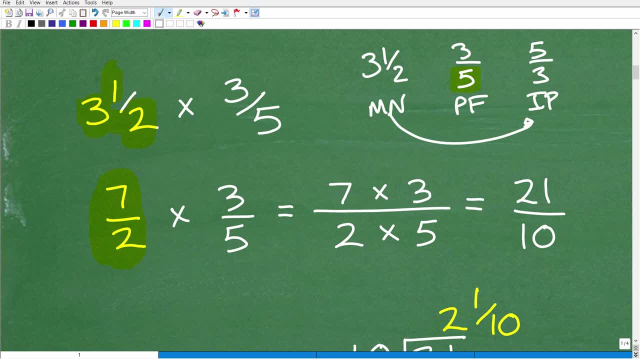 fractions. I have additional videos on this. I teach all of this in my pre-algebra course and my math foundation course. You can check those out by just going to my math help program. But let's go ahead and keep this problem going. So the first thing you're going to do, 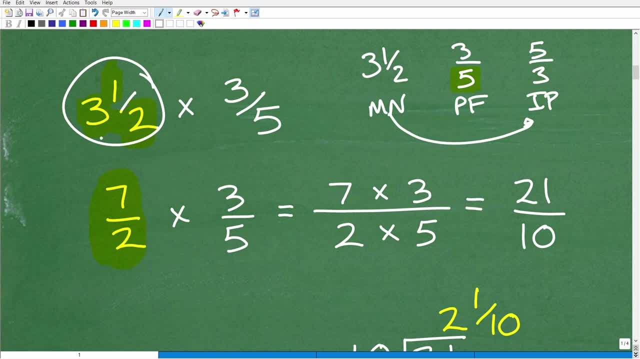 is you're going to multiply the number fractions into improper fractions. So that's going to be seven halves times our three fifths. So now we have one numerator, one denominator. one numerator, one denominator, And at this point we're good to go to go ahead and actually multiply the. 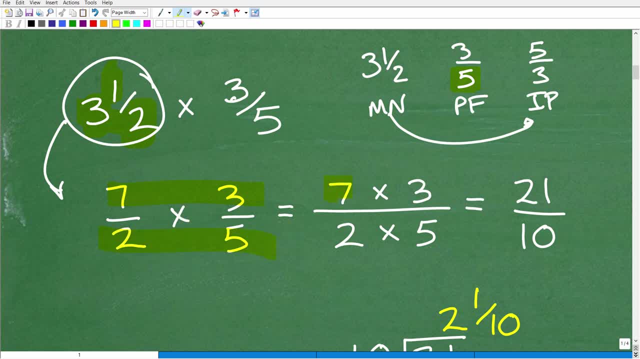 respective numerators and denominators. So seven times three. always write your factors out like this And I'm going to show you why here in a second: So seven times three. just don't answer that. It's going to be like: oh, seven times three is 21.. Show your work for. 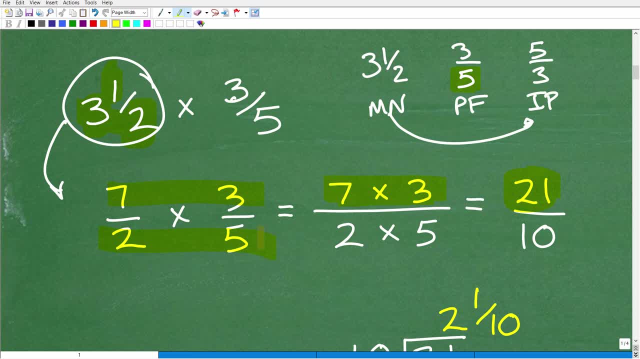 your teacher. But there's another reason here. in a second I'll show you. Of course, two times five is 10.. But you want to write it like this, because here I have seven times three and two times five. The reason why you want to write out all your factors here is because you want to look for. 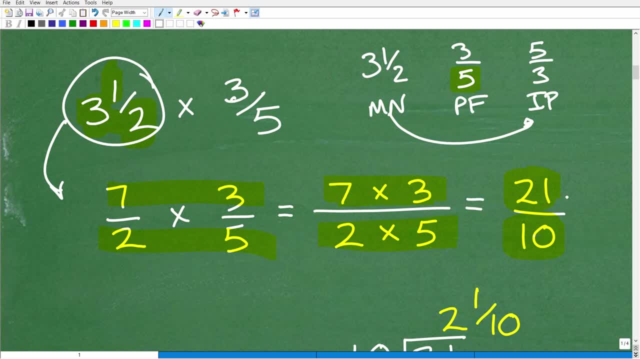 opportunities for cost canceling. So you can make sure that this fraction here is fully simplified. So two can't go into three, five can't go into seven, So all these numbers here are prime. So this answer is fully simplified. Now one thing. 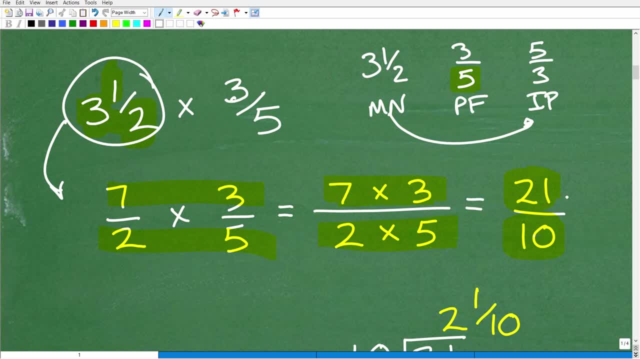 opportunities for cost canceling. So you can make sure that this fraction here is fully simplified. So two can't go into three, five can't go into seven, So all these numbers here are prime. So this answer is fully simplified. Now one thing. 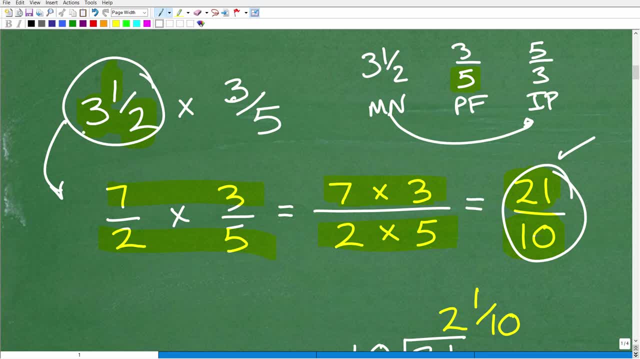 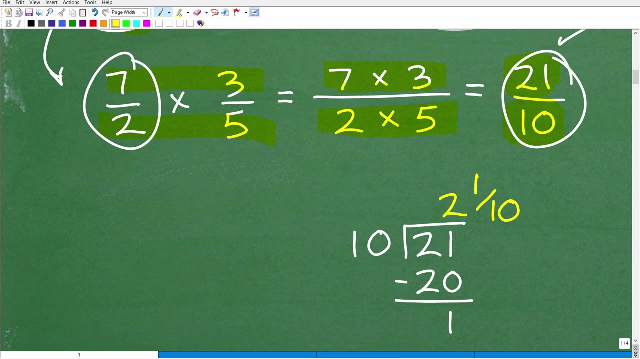 that we just did here is we took a mixed number and we wrote it as an improper fraction. We went from a mixed number to improper fraction. But you can also go from an improper fraction to a mixed number. You need to know how to do that, And the way that's done is you simply. 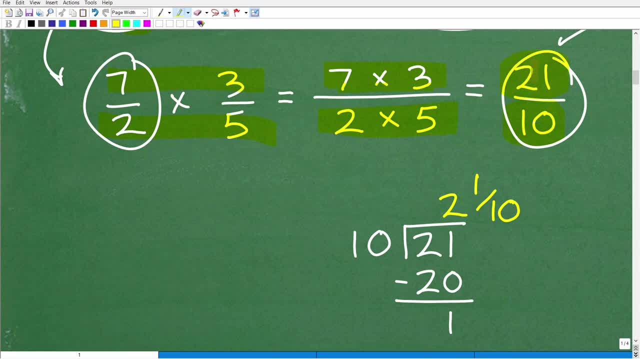 take your numerator. If we're dealing with an improper fraction, we take our numerator and we divide it by the denominator. So 21 divided by 10 is going to be, of course, 10 goes into 21, two. So two times 10 is 20.. So that's a remainder one, And then we're going to put that over this number. 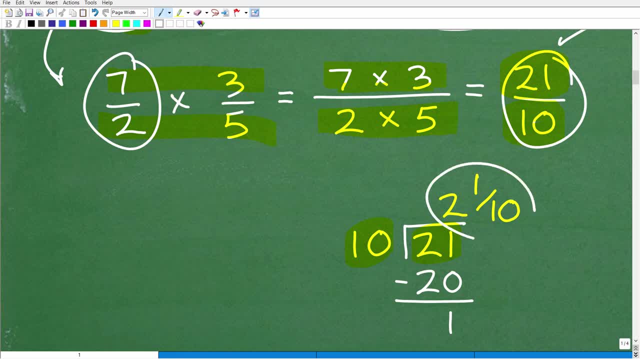 here 10.. So 21 tenths is the same thing as two and one tenths. Now I'm going to give you a really, really good piece of advice right here that will save you a lot of points on quizzes and tests. 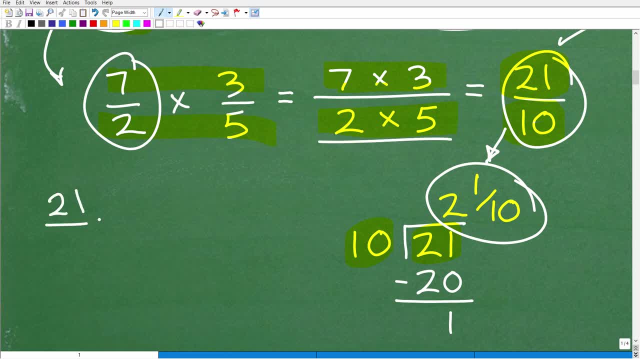 If you did this problem correct and a final answer is 21 tenths, and it's fully simplified. do not convert this into a mixed number fraction unless you are told to on by your teacher or the quiz or test exams. OK, don't take the initiative and do the extra work. There's two. 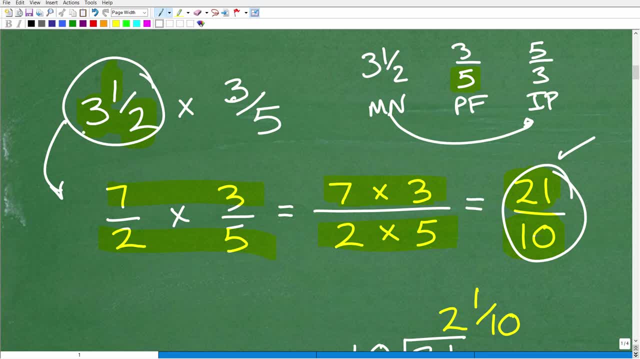 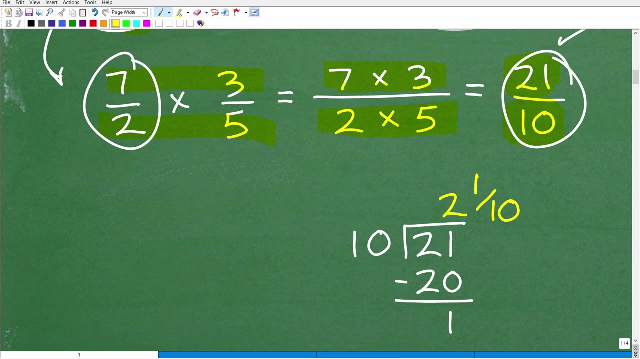 that we just did here is we took a mixed number and we wrote it as an improper fraction. We went from a mixed number to improper fraction. But you can also go from an improper fraction to a mixed number. You need to know how to do that, And the way that's done is you simply. 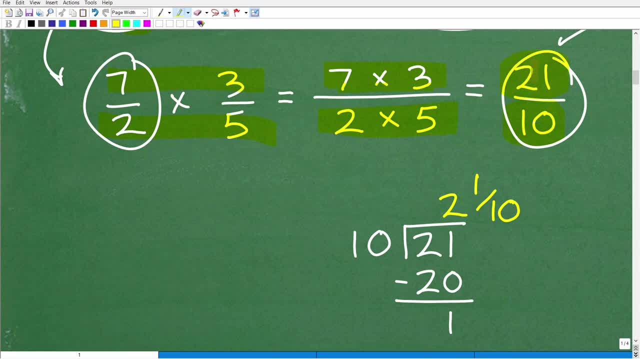 take your numerator. If we're dealing with an improper fraction, we take our numerator and we divide it by the denominator. So 21 divided by 10 is going to be, of course, 10 goes into 21, two. So two times 10 is 20.. So that's a remainder one, And then we're going to put that over this number. 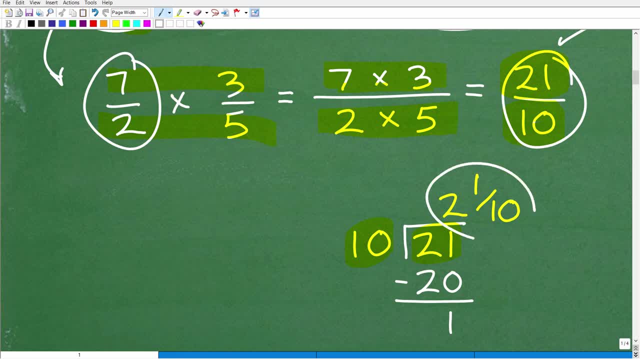 here 10.. So 21 tenths is the same thing as two and one tenths. Now I'm going to give you a really, really good piece of advice right here that will save you a lot of points on quizzes and tests. 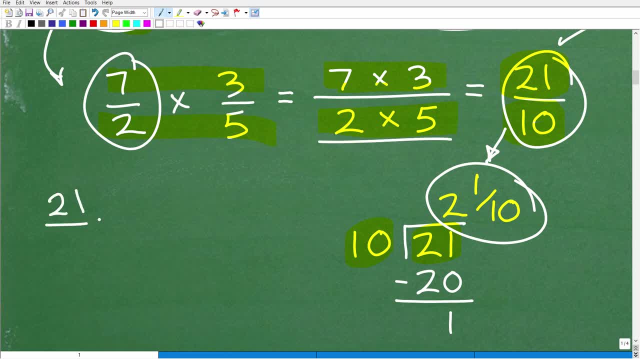 If you did this problem correct and a final answer is 21 tenths, and it's fully simplified. do not convert this into a mixed number fraction unless you are told to on by your teacher or the quiz or test exams. OK, don't take the initiative and do the extra work. There's two. 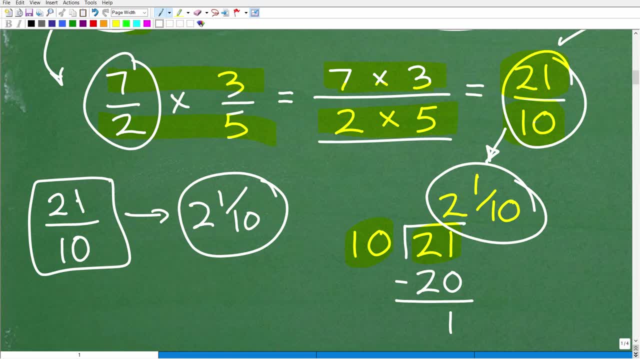 reasons why: One, it's going to take you time to write 21 tenths as a mixed number. two, and one tenths, It's going to take you additional time on your test or quiz. And two, I've seen thousands upon thousands of times that you can write 21 tenths as a mixed number, So 21 tenths is going to. 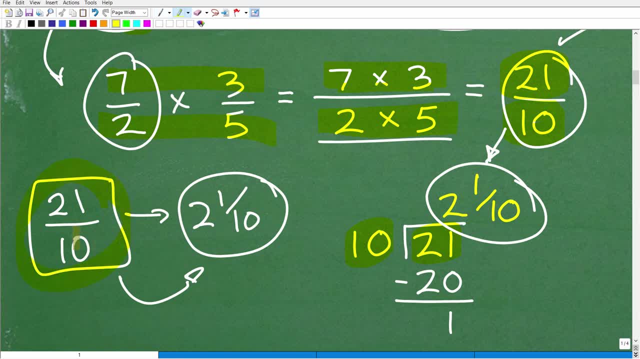 take you thousands of errors where the student actually had the right answer. But then you went to go do this division and then they messed this up. They write like two and one eighth or they make some sort of mistake and then they turn this answer in and then you got to mark it down And 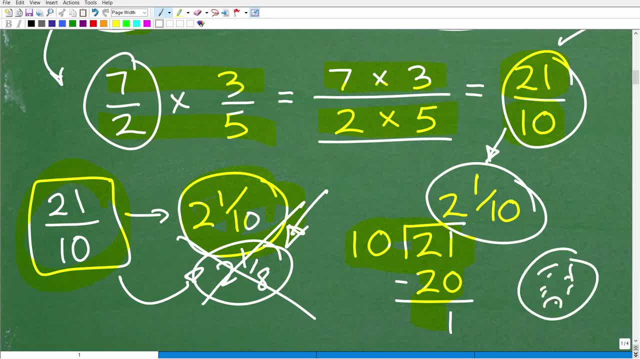 then there's a lot of- like you know- sad faces with tears and everything else, And nobody likes that. So here's the deal. OK, unless you're told to again write your final answer as a mixed number fraction, do not do it. 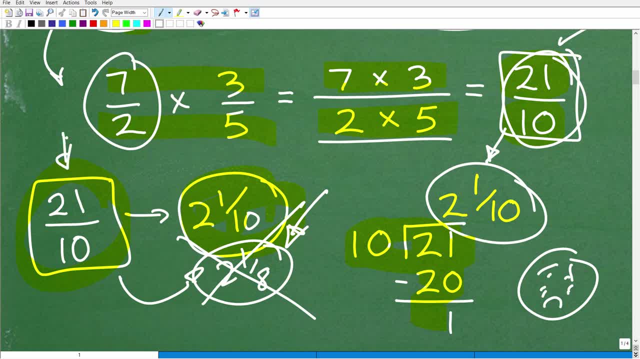 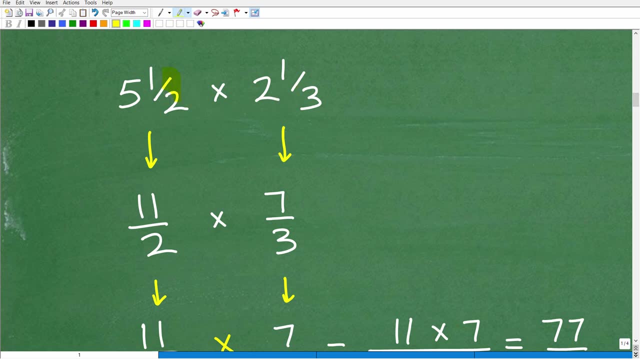 However, you do need to make sure you all your answers when it comes to fractions- whether you're adding, subtracting, multiplying, dividing- are fully simplified. OK, so let's go and take a look at one more situation- And this is just more review with mixed numbers. So here we have five and one. 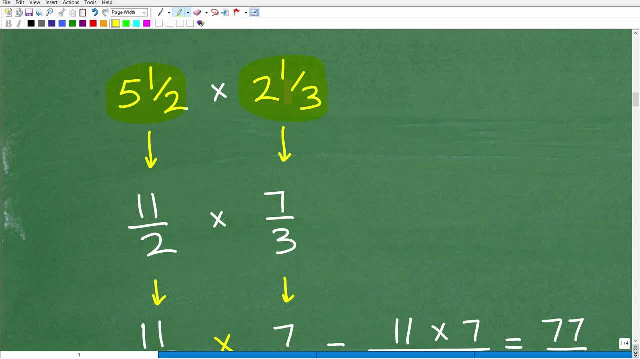 half times two and one thirds. Again, we can't multiply mixed in mixed number form, So we want to go ahead and change those into improper fractions. So here this would be a little bit more complicated. So here we have: two times five is ten plus one. That's going to be eleven or eleven. 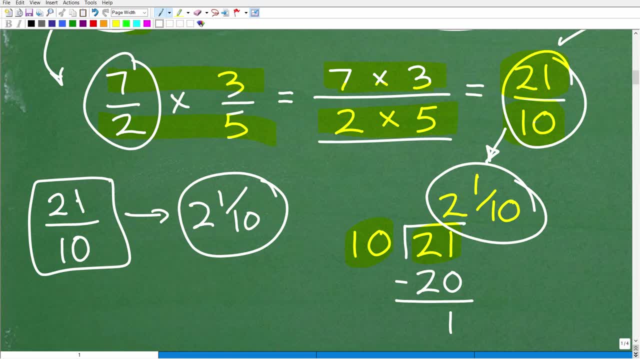 reasons why: One, it's going to take you time to write 21 tenths as a mixed number. two, and one tenths, It's going to take you additional time on your test or quiz. And two, I've seen thousands upon thousands of times that you can write 21 tenths as a mixed number, So 21 tenths is going to. 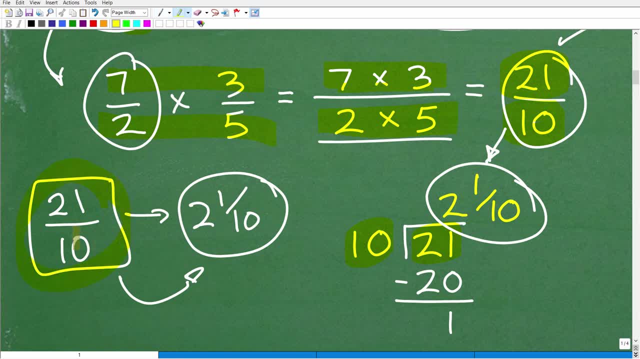 take you thousands of errors where the student actually had the right answer. But then you went to go do this division and then they messed this up. They write like two and one eighth or they make some sort of mistake and then they turn this answer in and then you got to mark it down And 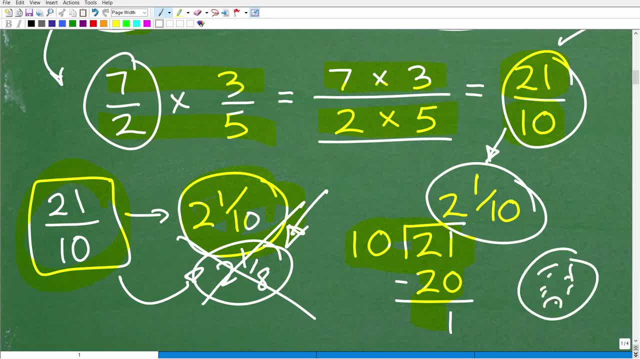 then there's a lot of- like you know- sad faces with tears and everything else, And nobody likes that. So here's the deal. OK, unless you're told to again write your final answer as a mixed number fraction, do not do it. 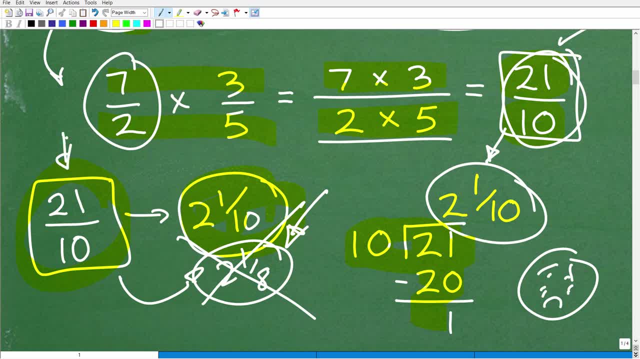 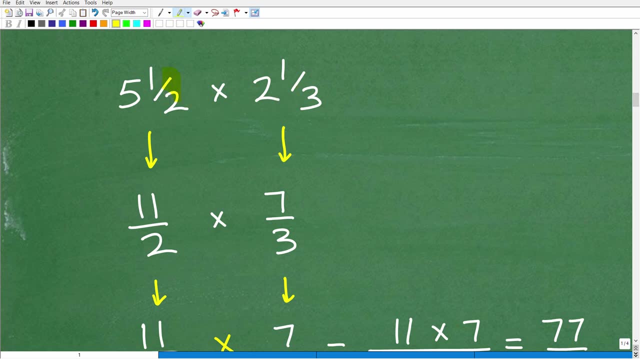 However, you do need to make sure you all your answers when it comes to fractions- whether you're adding, subtracting, multiplying, dividing- are fully simplified. OK, so let's go and take a look at one more situation- And this is just more review with mixed numbers. So here we have five and one. 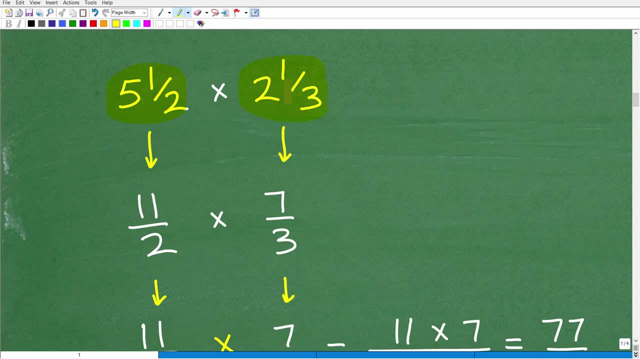 half times two and one thirds. Again, we can't multiply mixed in mixed number form, So we want to go ahead and change those into improper fractions. So here this would be a little bit more complicated. This would be: two times five is ten plus one. That's going to be eleven or eleven. 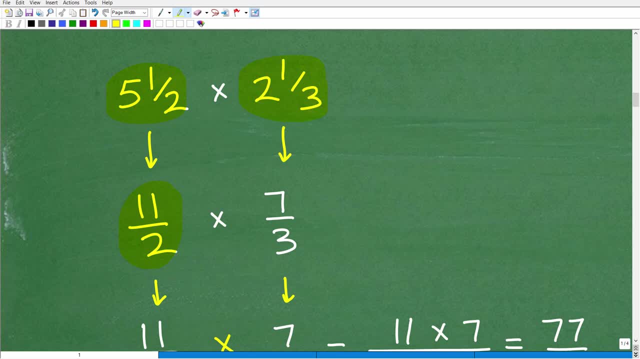 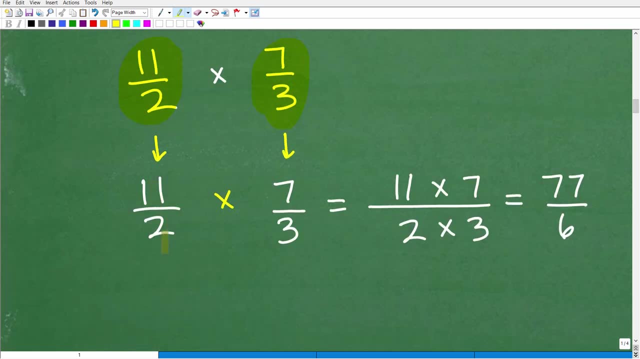 halves. here This would be three times two is six plus one is seven or seven thirds. So now I want to go ahead and do the problem: Eleven halves times seven thirds. So here it is: Eleven halves times seven thirds. Again, I'm going to multiply the respective numerators and denominators, So eleven. 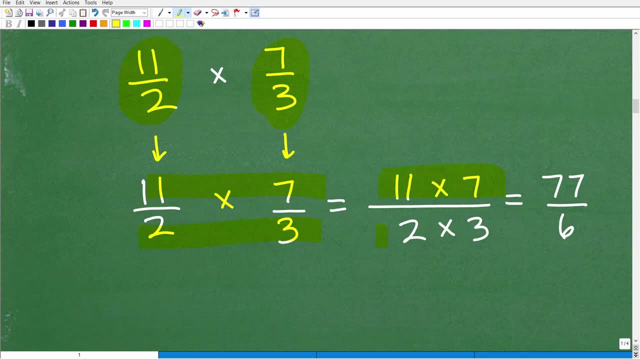 times seven. I'm going to write the factors out this way: Two times three is like is two times three, And I'm looking for opportunities to cross cancel And these are all prime numbers. So let me go ahead and do the actual multiplication Eleven times. 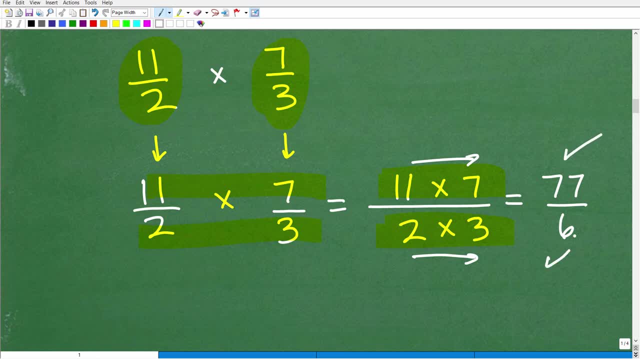 seven is seventy seven and two times three is six, And I could be 100 percent confident that that answer is fully simplified. Again, you don't have to question whether this answer is fully simplified. if you kind of took a look at the factors and you look for opportunities to cross, cancel, OK. 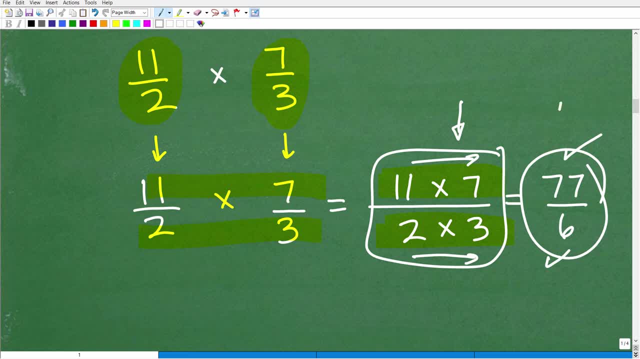 so that really really helps you out, Kind of like doing the work in advance And then you can just be fully confident that your answer is correct. OK, so we just covered how to multiply fractions. How did you do if you knew all this stuff and you're like this was just total review? 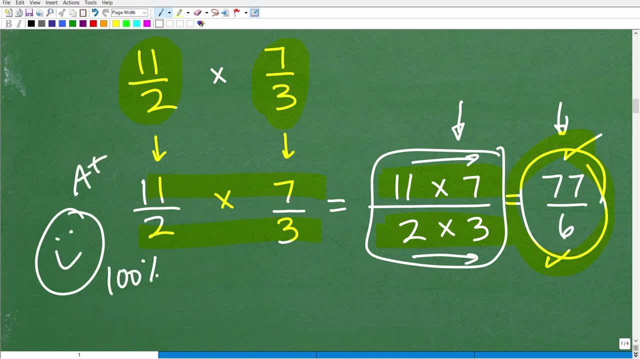 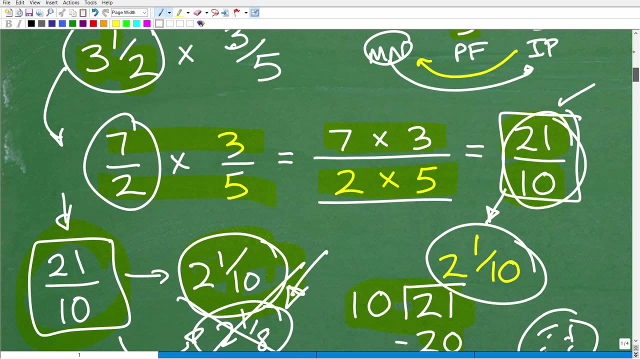 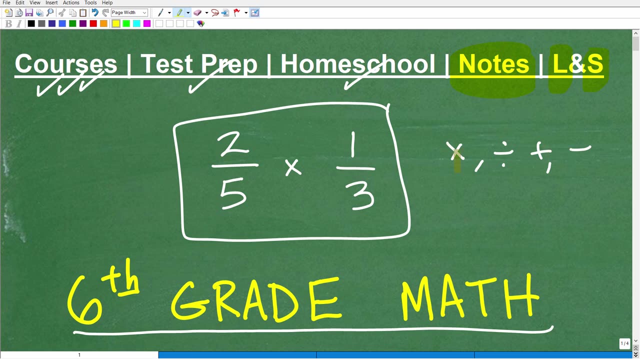 I must give you a nice little happy face and a plus one hundred percent and multiple stars so you can have a wonderful day. Nice job, OK. but again, remember, let's kind of go back up here And in the very beginning the easiest thing to do, to kind of learn about fractions. 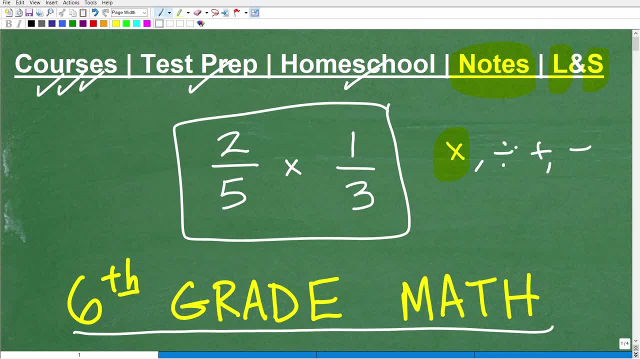 in my opinion, is how to multiply. OK now, you can't divide fractions unless you understand how to multiply fractions. So if you, kind of reviewing fractions, start with multiplication, then move on to division. What you're going to do with division of multiplication, I'm sorry, division problems of 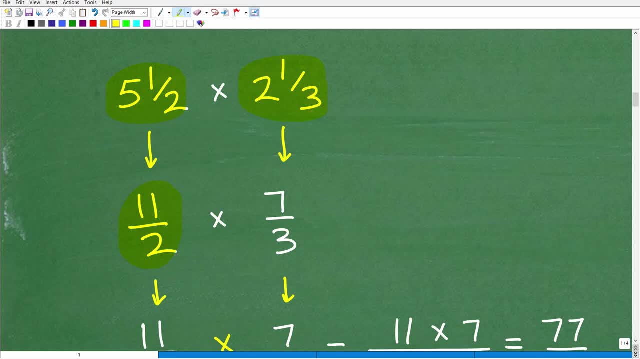 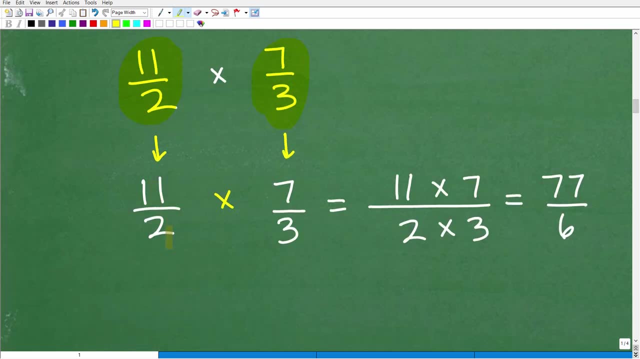 halves. here This would be three times two is six plus one is seven or seven thirds. So now I want to go ahead and do the problem: Eleven halves times seven thirds. So here it is: Eleven halves times seven thirds. Again, I'm going to multiply the respective numerators and denominators, So eleven. 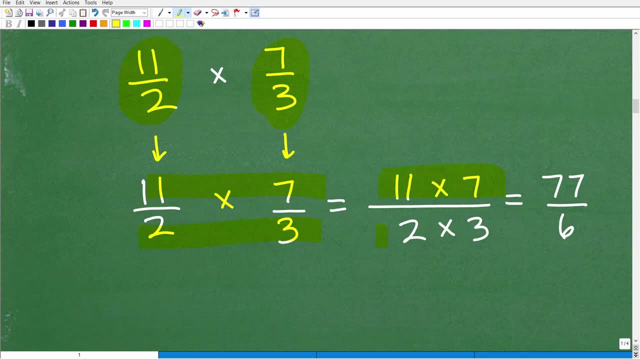 times seven. I'm going to write the factors out this way: Two times three is like is two times three, And I'm looking for opportunities to cross cancel And these are all prime numbers. So let me go ahead and do the actual multiplication Eleven times. 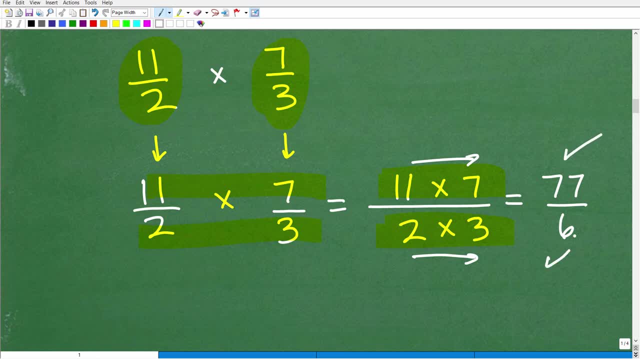 seven is seventy seven and two times three is six, And I could be 100 percent confident that that answer is fully simplified. Again, you don't have to question whether this answer is fully simplified. if you kind of took a look at the factors and you look for opportunities to cross, cancel, OK. 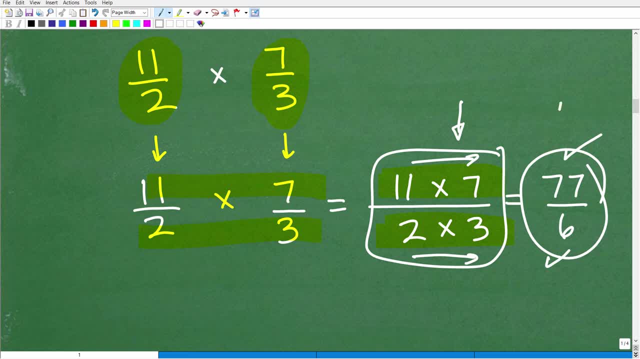 so that really really helps you out, Kind of like doing the work in advance And then you can just be fully confident that your answer is correct. OK, so we just covered how to multiply fractions. How did you do if you knew all this stuff and you're like this was just total review? 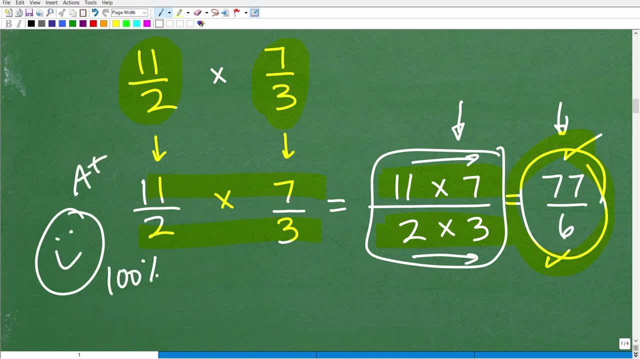 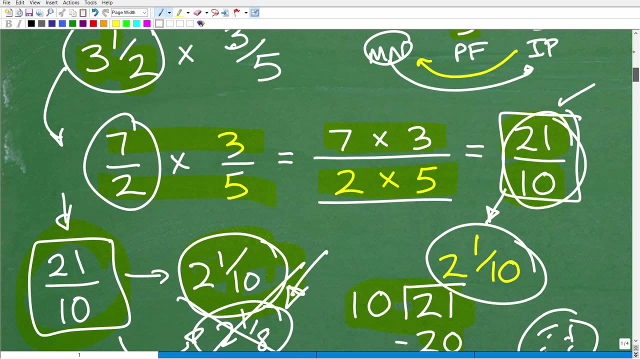 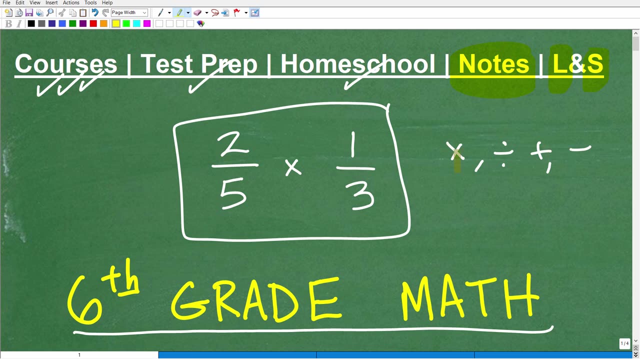 I must give you a nice little happy face and a plus one hundred percent and multiple stars so you can have a wonderful day. Nice job, OK. but again, remember, let's kind of go back up here And in the very beginning the easiest thing to do, to kind of learn about fractions. 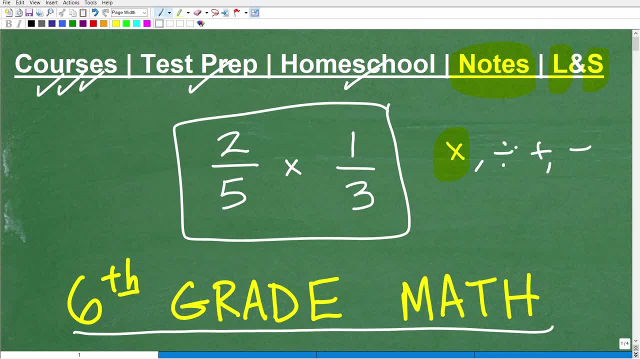 in my opinion, is how to multiply. OK now, you can't divide fractions unless you understand how to multiply fractions. So if you, kind of reviewing fractions, start with multiplication, then move on to division. What you're going to do with division of multiplication, I'm sorry, division problems of 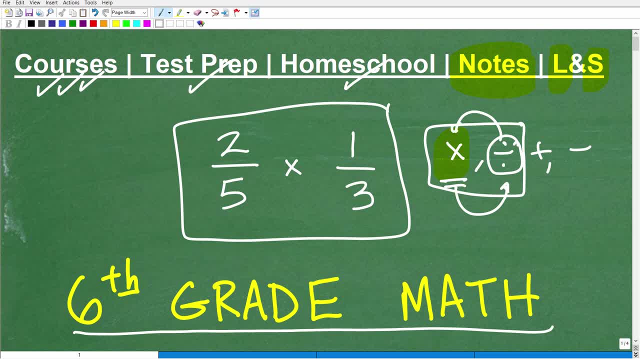 fractions. excuse me, is you're going to convert division problems into multiplication problems? So all this right here is really just multiplication And you're talking about two of the operations that we do in mathematics, And when it comes to fractions, is super easy, OK, multiplying. 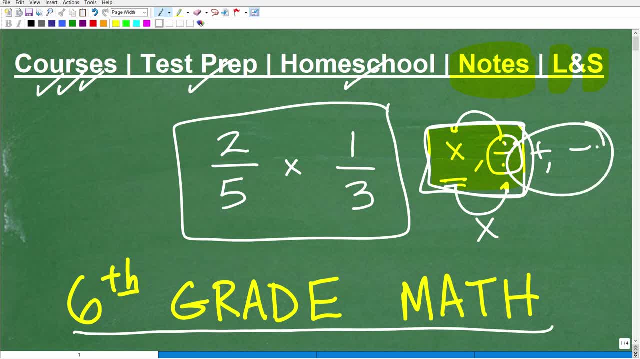 and dividing fractions: Easy, easy, easy. But when it comes to addition and subtraction, this is where students kind of like panic because they're like, oh no, I got to find the LCD. Well, you got to check out some of my videos on fractions. A matter of fact, I have one or two, maybe even more than.